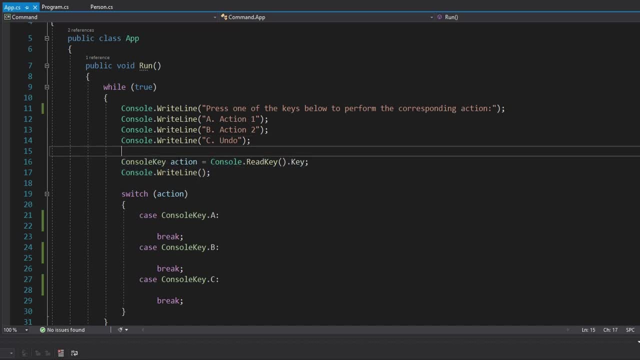 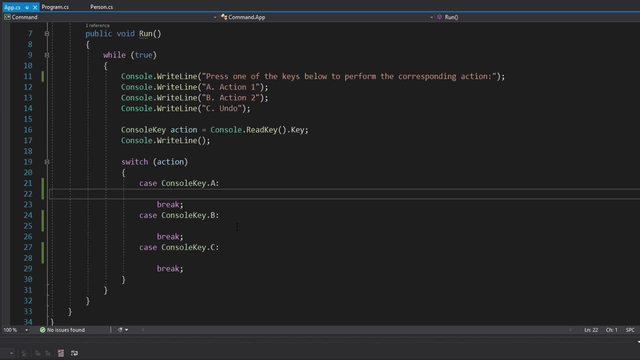 undo operation, So we figure out what the user typed in, and then we're going to perform the corresponding operations inside of this switch statement. Now, the key here is that this user interface is intended to support hundreds of applications, so that's like the constraint we're going to enforce. 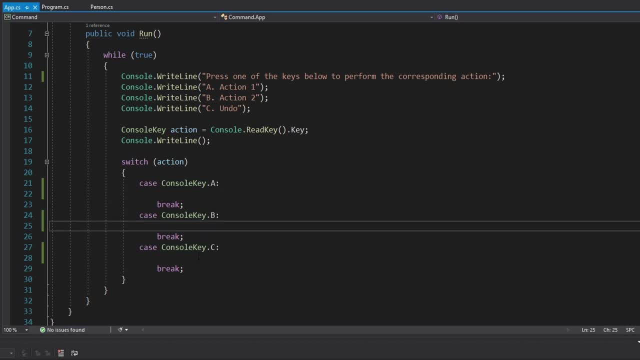 here, So we can't just hard code all of our behavior inside of this switch statement. we want this to be reusable, So instead, what we're going to do is implement the command pattern. So we're going to depend on an I command interface, which we're going to implement in just a second. 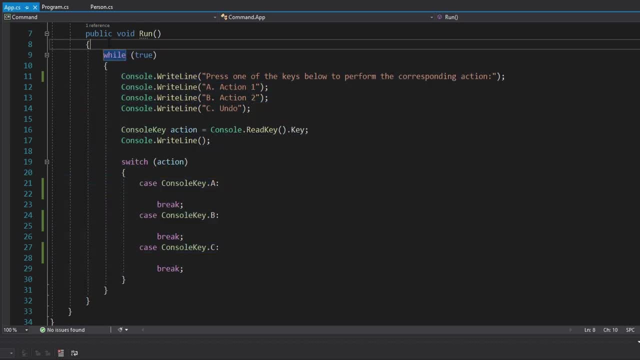 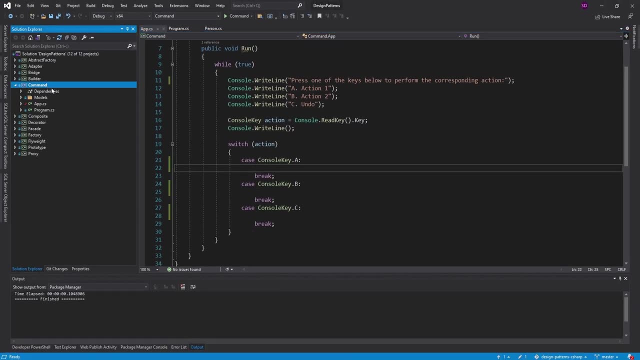 and every other application that wants to use this user interface can just pass in any commands that we want and it'll work flawlessly. So let's go ahead and first set up our commands. So first we're going to create that I command interface. I'm going to put all of this into a commands. 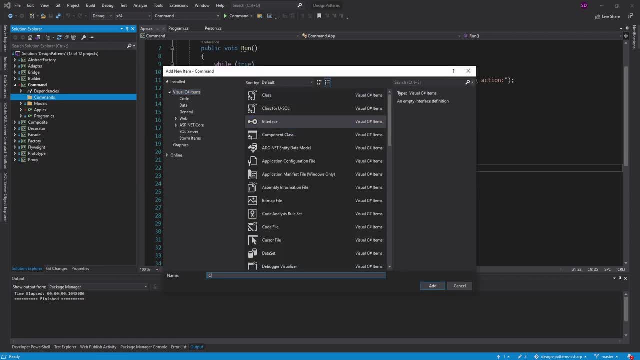 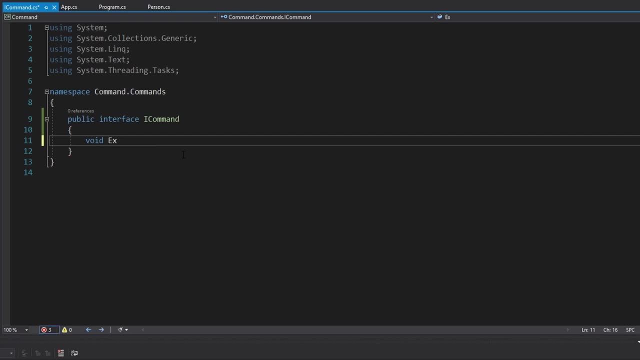 folder. So we're going to have an interface. this is going to be an I command- And on this interface we're going to have a single method. it's going to be a void because we don't need to return anything. we're going to call it execute. So just a general name here and not going to pass. 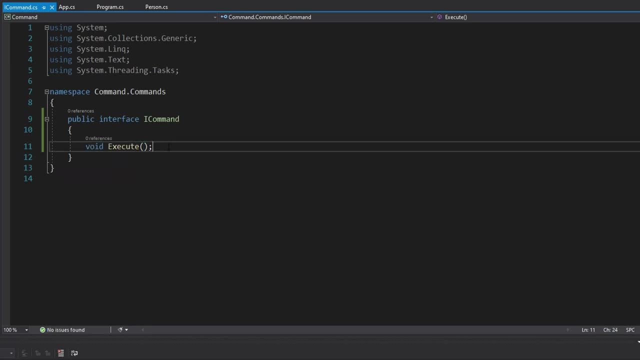 in any parameters. So again, no return type, no parameters. all this interface is really doing is connecting our user interface to our applications behavior. So, that being said, there really shouldn't be anything to return And there shouldn't be anything that we pass into this. 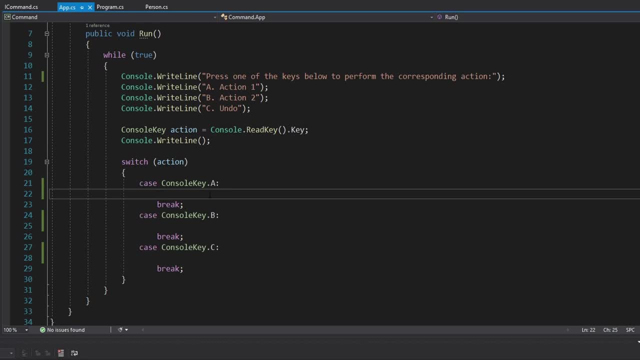 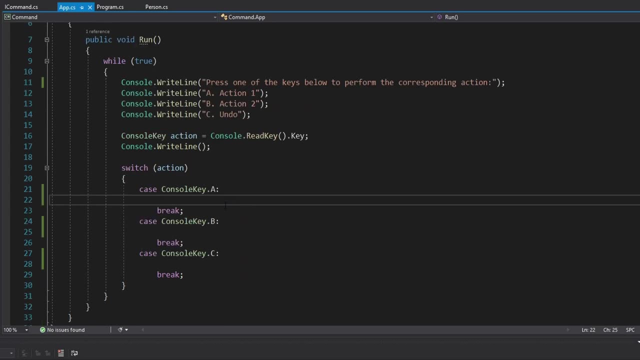 method. all that's going to happen is that we're going to execute a command whenever the user presses one of these console keys. So now that we have our interface, let's go ahead and depend on that I command interface. So we're going to have three fields in here. we're going to get three. 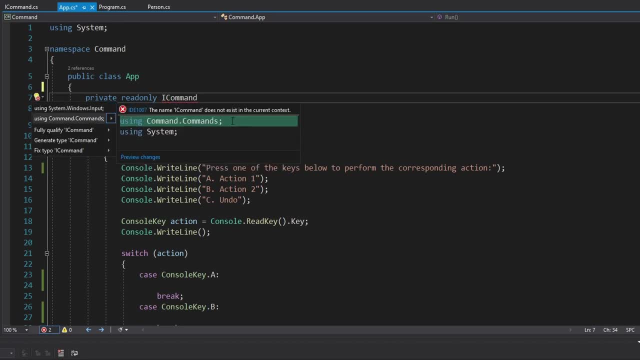 commands passed in and make sure you import our command interface, because there is one in system that windows, that input, And that's the one that we use for things like WPF. I actually use it all the time, But I figured we create our own And again I'm going to have commands for each of our 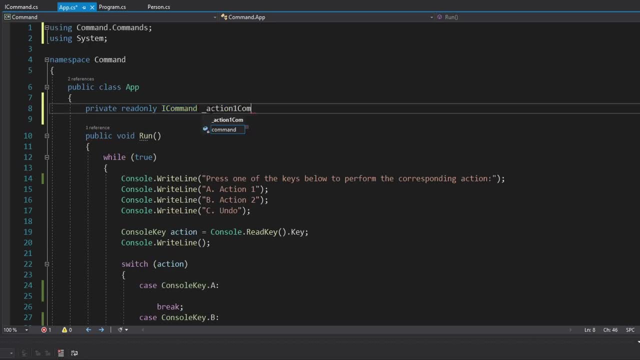 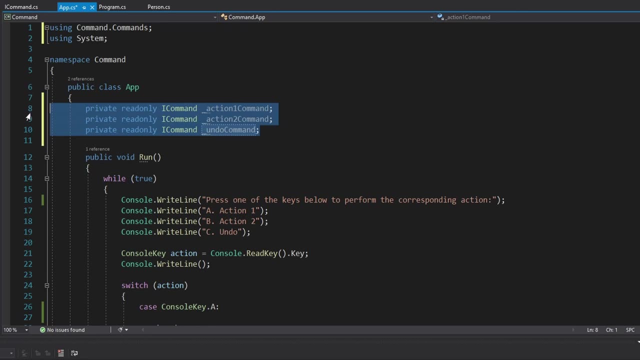 actions. So this is going to be action: one command and then two more action to command, And then finally our undo commands, And let's just get these passed through the constructor, And now we'll have these commands initialized, And then we're going to have these commands pass through. 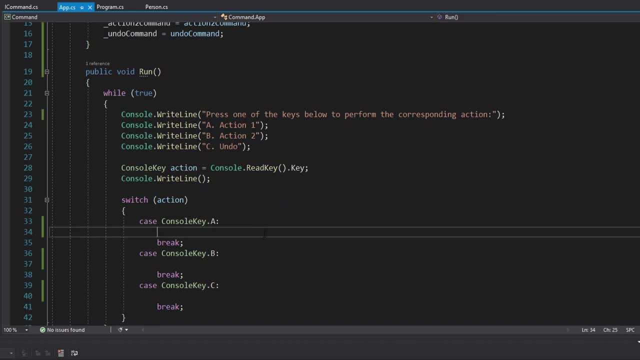 the constructor, And now we'll have these commands initialized, And now we'll have these commands passed through the constructor, And then we'll have these commands pass through the constructor. So let's hook those up to our console keys. So console key A is going to perform action one. So 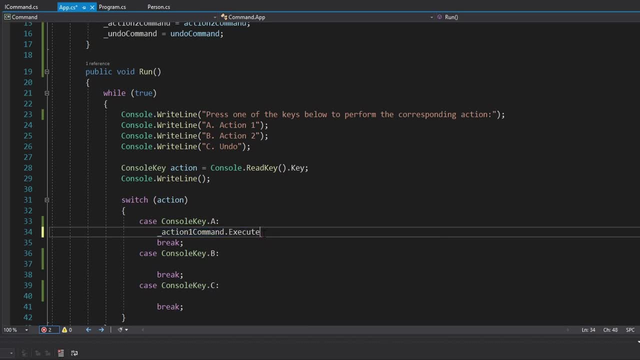 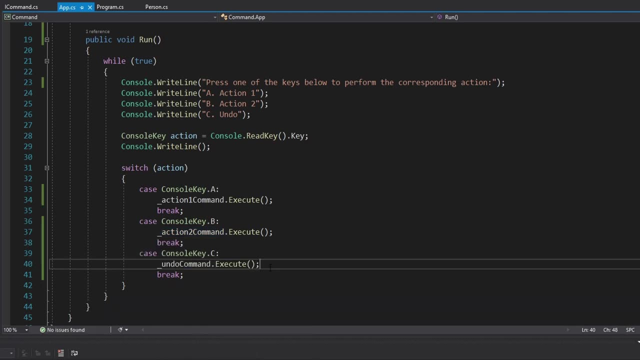 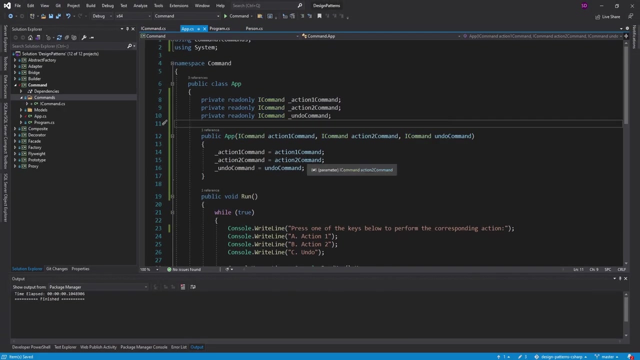 we'll take our action one command and execute that, and then similar for console key B, except this is action, two commands, and then C is going to be our undo commands. So now our user interface depends on these commands And we can pass in any commands that we want into our user interface. But first: 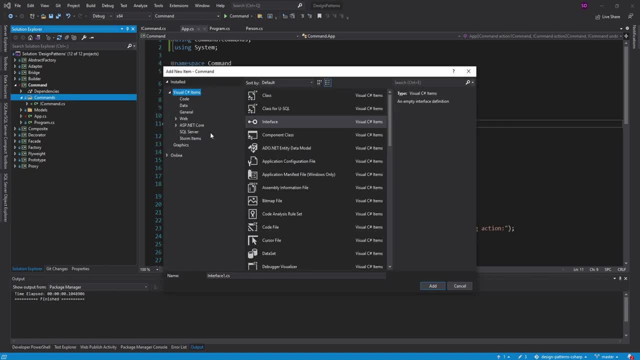 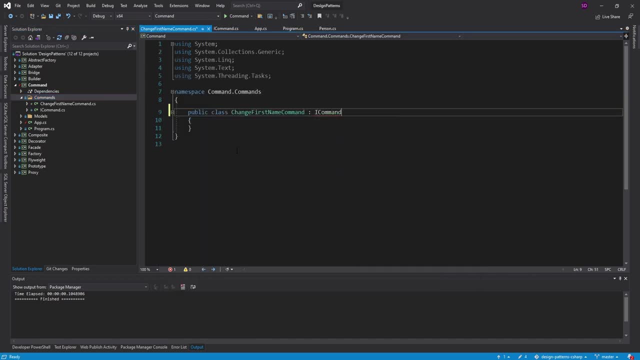 we're gonna have to actually implement a command. So let's create a new class. I'll call this the change first name command And it's going to implement our new I command interface. So implement that. And the reason I chose change first name as the name of our command is because 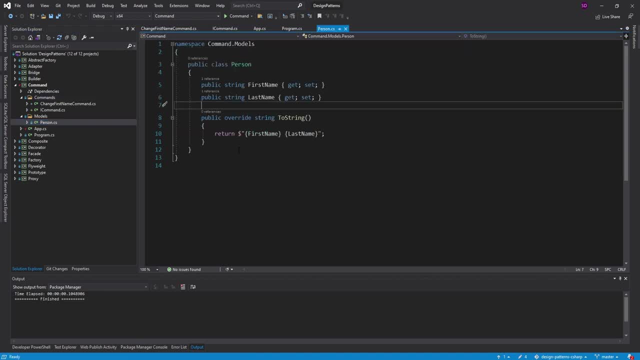 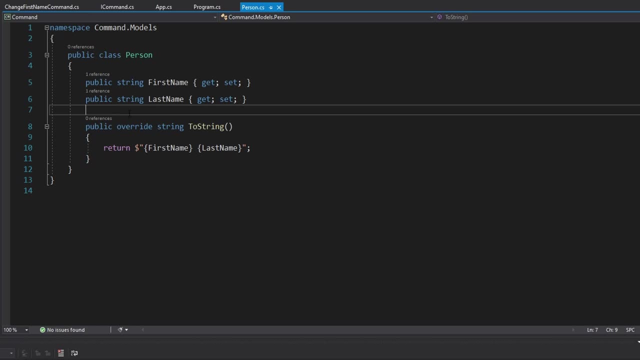 I actually have this model over here for a person, So this is what we're going to be using to implement some logic in our application. Just a simple class with a first name, a last name and an override on to string that prints out their first name and last name. So nothing. 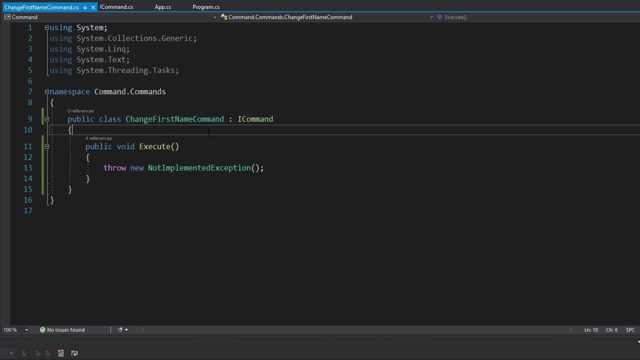 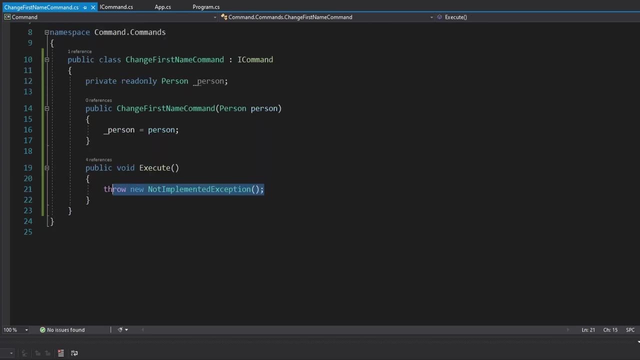 crazy there. But we are going to have a command to change that person's first name. So let's get that person passed in here, So I'm going to put that in a field and get that through the constructor And then all we're going to do and execute is take that person And we're going to 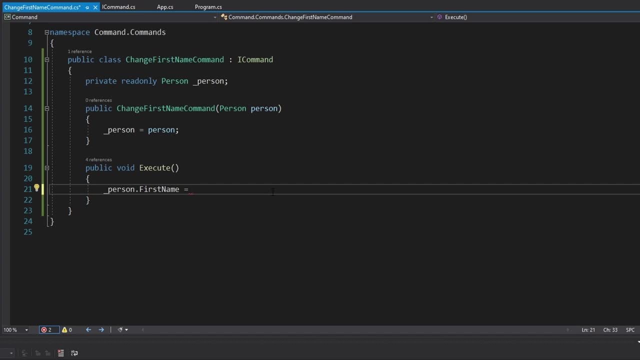 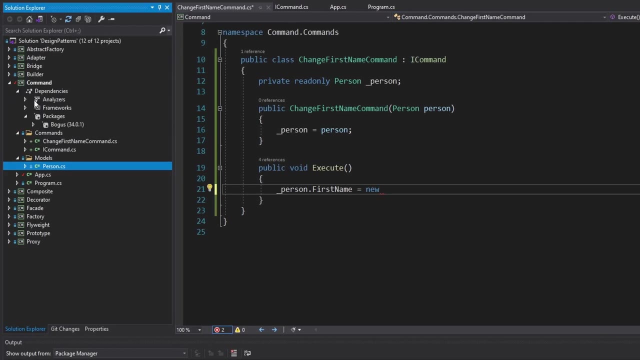 change their first name And we're just going to generate a random first name. So I'm going to use bogus for this, which is a useful package to generate fake data, And I think I already have this installed. So packages, we have bogus, So make sure you grab that off nougat if you're using. 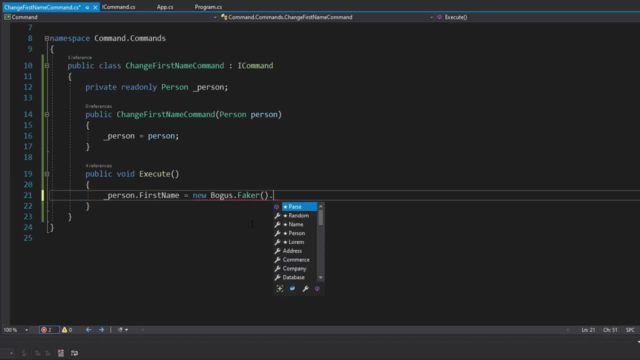 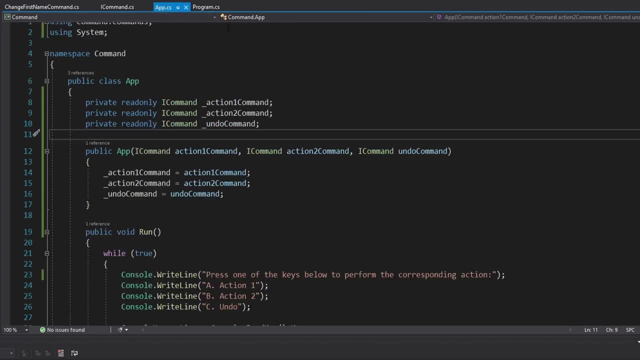 it here, But we're going to instantiate a new bogus faker And we're just going to dig into that person and grab a random first name. So let's pass this command to our app And that's going to be done in our programcs. So we have to pass in three commands. we're going to have the. 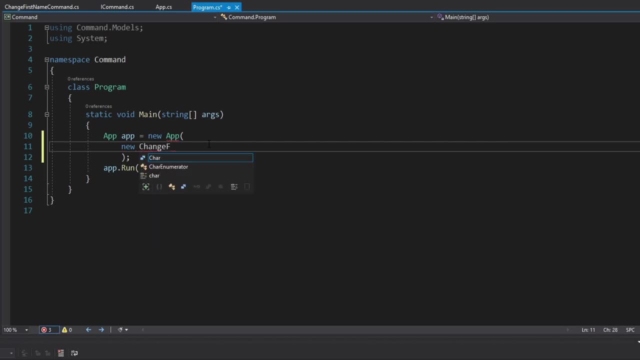 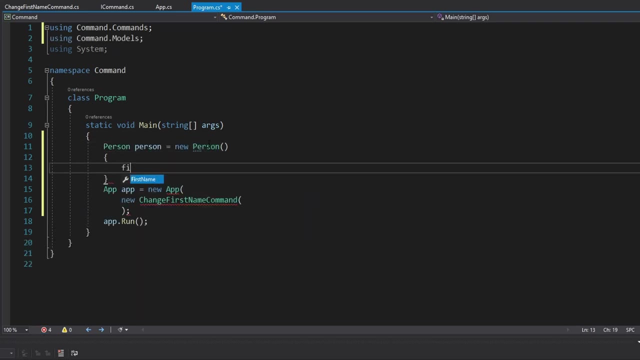 change first name command as action one. So let's instantiate that here. And then we're going to have to instantiate a person. Let's do that up here as well. new person and their initial first name will be singleton And last name will be Sean. So let's pass that person to our command. 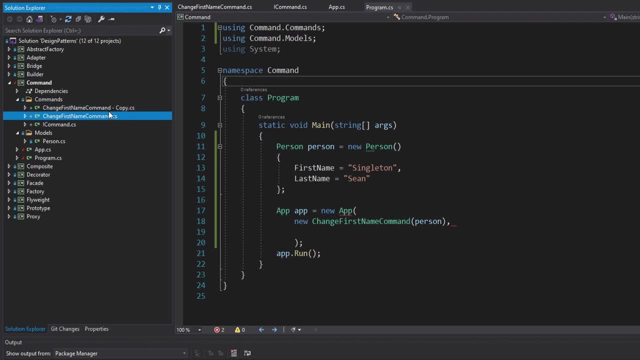 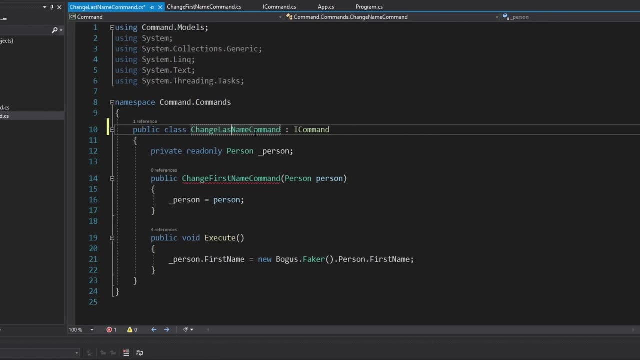 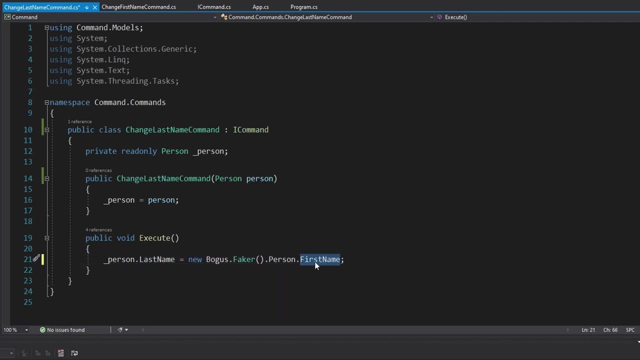 And now we need an action To command, So it's going to copy this first one and rename this to be the change. You guessed it. change last name commands to make sure we fix that inside of here. change last name commands And now we're just going to set the person's last name to a random last name from bogus. 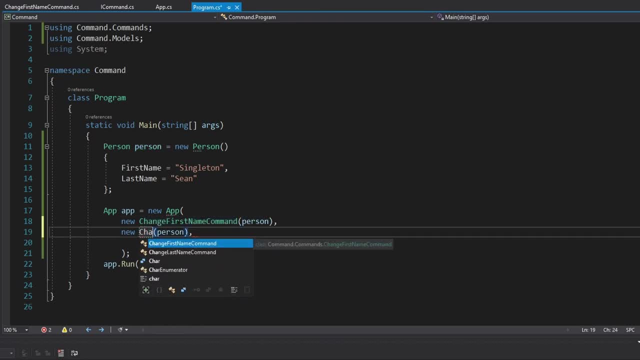 And then let's pass that to action two, So the change last name commands and actually we'll implement the undo stuff next. But first I want to test this out, So let's just pass in null for the do commands. And then, lastly, if we want our application to be useful, So we can actually 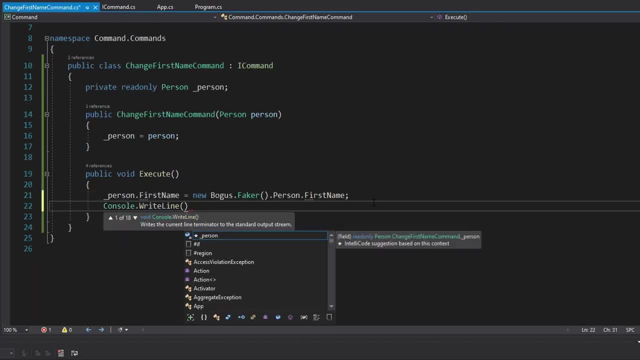 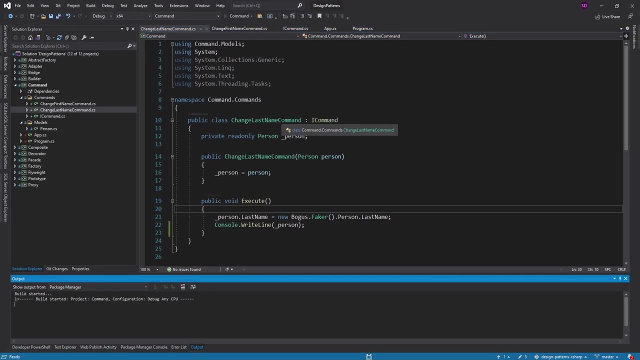 see what's going on. Let's console Rate Line are person after we change anything on their name, And let's do that for both of our commands. So let's go ahead and run this and we should get what we expect. So let's press a and we changed our first names. Then we have Carlton Sean. 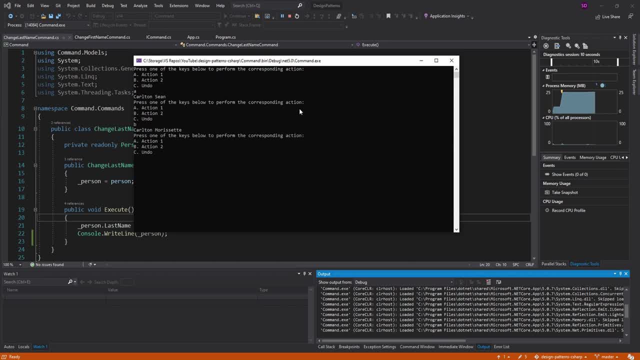 Let's change our last name. Now we have Carlton Dennarius. Cool, I didn't think I'd be getting names Carlton, please, And or set. I think that's That's your name, CarltonI don't. I didn't think I'd be getting hard names. Carlton Morissette- I think that's your name, Carlton, And then. 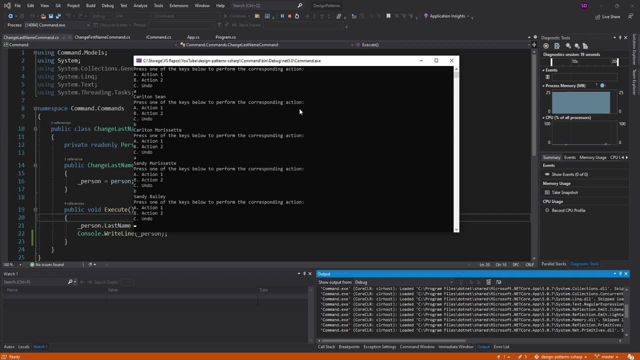 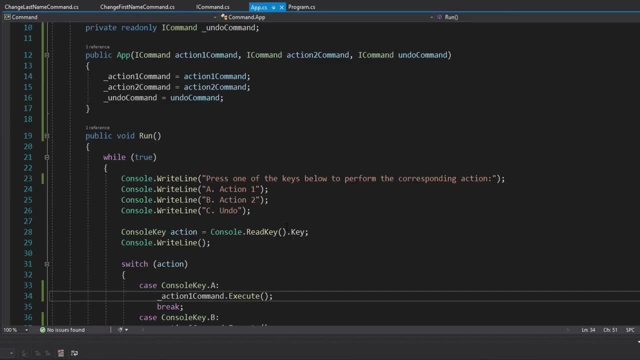 Carlton ook feel praying for love when I go at Charlie's birthday party. mean name more a set. I think that's right. But yeah, it looks like it's working as expected And the key here is that our user interface is just dependent on these commands. So if we ever want this UI to 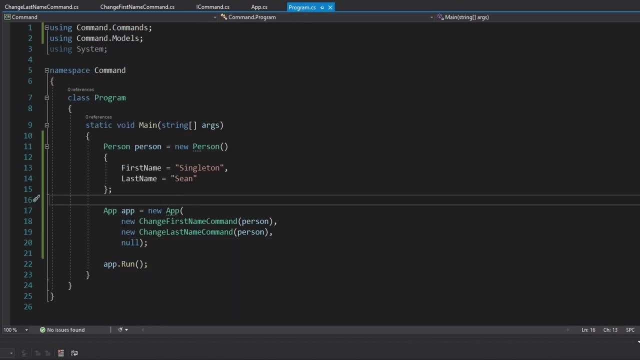 do something else. all we have to do is pass in different commands to our app. And just to relate this to other technologies, this is how WPF commands work as well. So if we recall buttons in WPF, they have a command property on them And that command property takes in an I command. 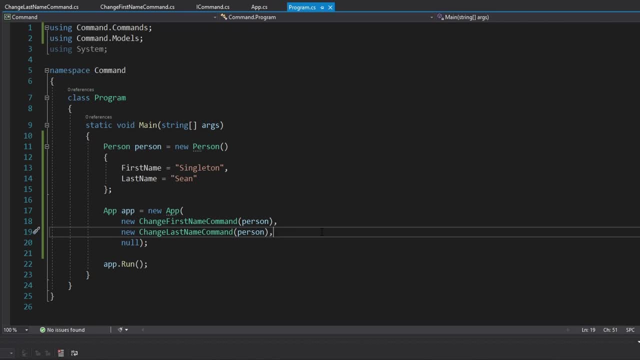 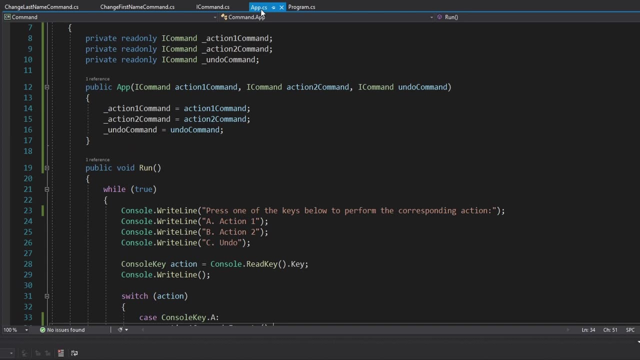 And my application, your application, everybody's application can just pass in any command that they want, as long as it satisfies the I command interface. So that's essentially the same thing we're doing here, except my user interface probably isn't going to be reused by anyone. 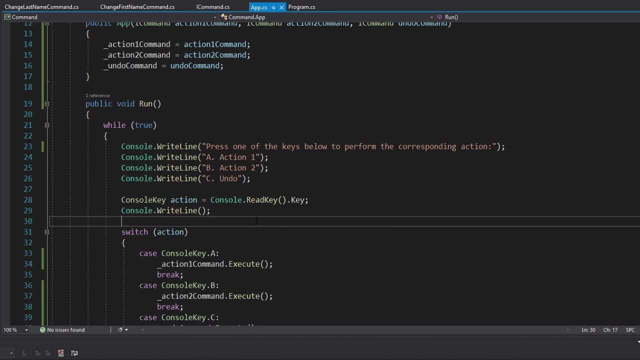 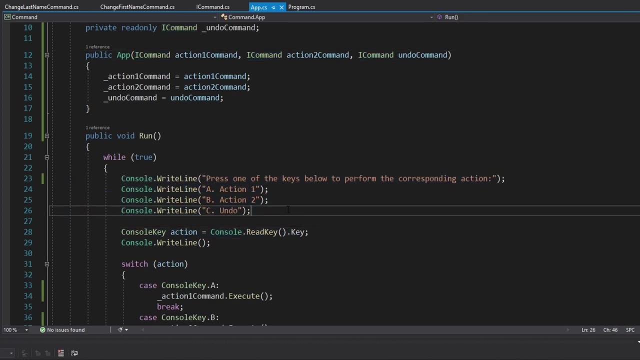 at least not on the scale that a WPF button would be. But anyways, we've covered this idea of depending on an I command interface, so that the client or the user interface can support various commands without having to change. But now let's get into this undo concept. So since 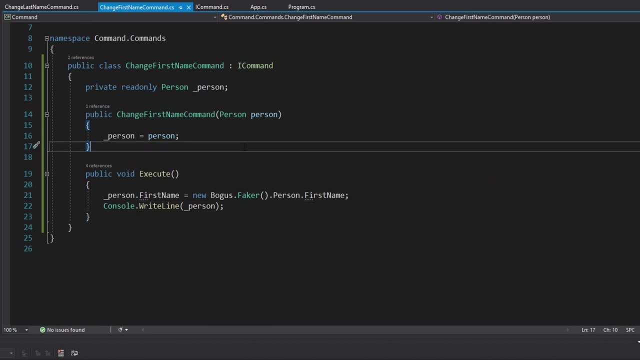 our command is wrapped inside of a class. we could store some data inside of this class to support undoing the operation. So in order to undo changing the person's first name, we're first going to have to figure out what their previous first name was. So we're going to store. 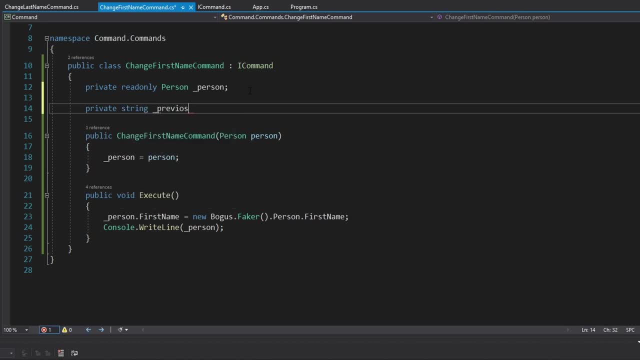 that inside of a field. So let's get a string up here. we'll call this previous first name And then we'll just set this before we change their first name, And we're going to set it to the person's current first name. And now, if we want to undo this command, so let's add an undo method. 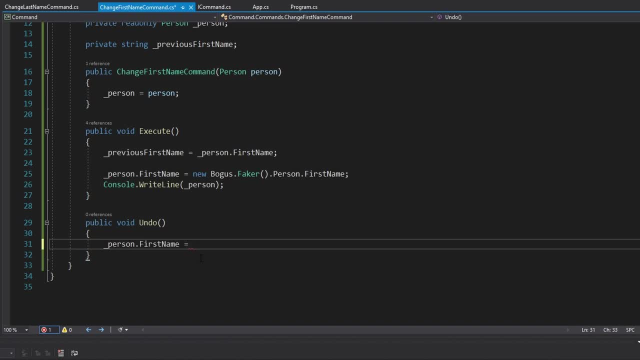 all we have to do is set the person's first name to the previous first name, And actually maybe we should only do this if the previous first name is not null. So let's have that little check in there, Because if we never execute this command, then the previous first name is. 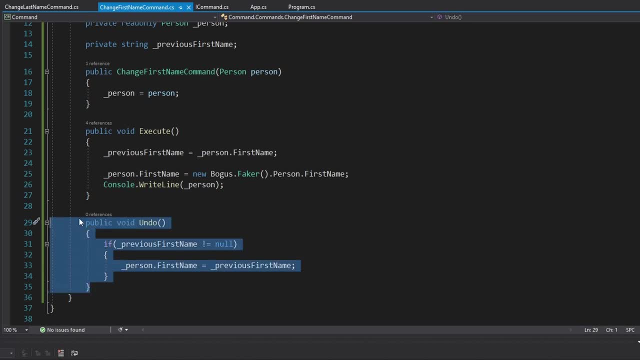 going to be null. But anyways, let's go ahead and move this over to the change last name command. So just gonna pretty much copy paste this, Except this is not going to make any sense because there's going to be a couple of things that we need to fix in here. But yeah, basically the first name is going to be null. Sof, we're. 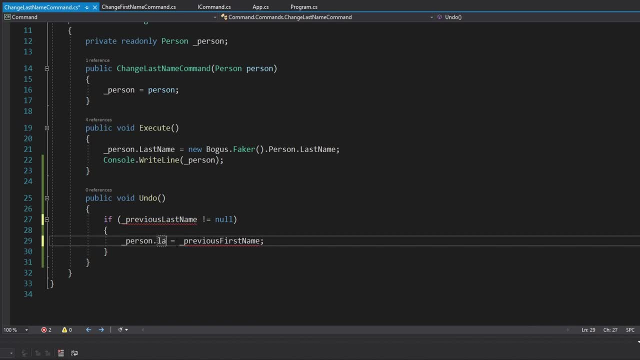 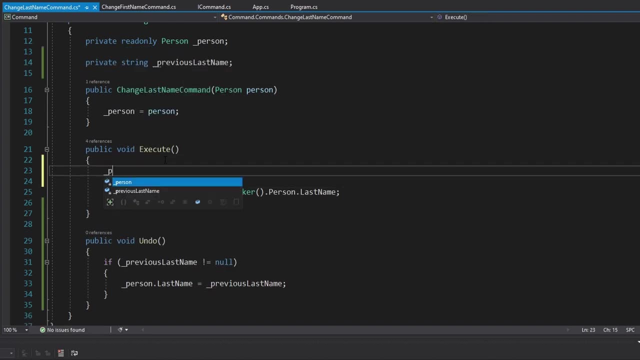 now going to be previous last name and we're going to be changing the person's last name again, and then let's add this field. it's going to be a string and then we're going to set previous last name. so now we support undo on these commands, but first we're going to have to actually have an undo. 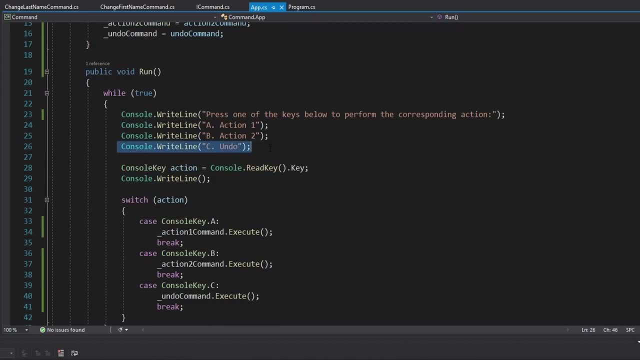 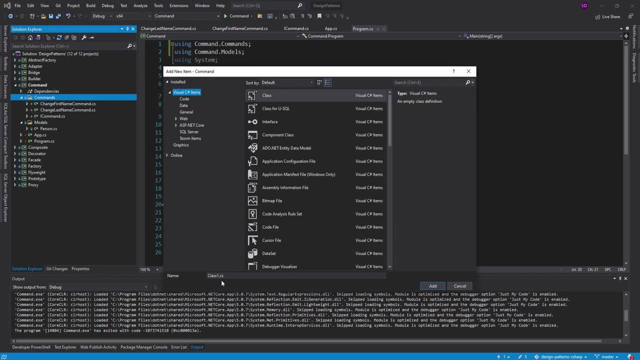 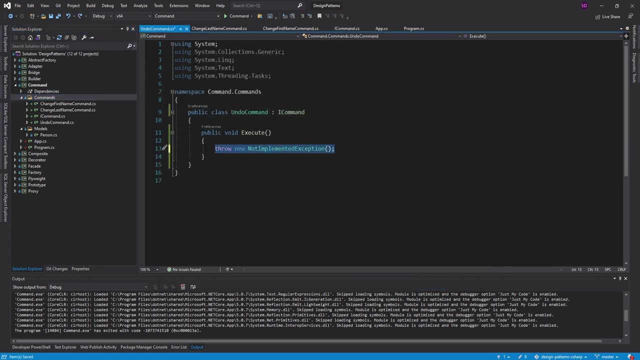 command that we can pass into our user interface, because right now undo command we pass as null, so let's add that command. this is going to be a new item here, the undo command. it's going to implement our i command interface and all we're going to do in here is undo the commands. but what? 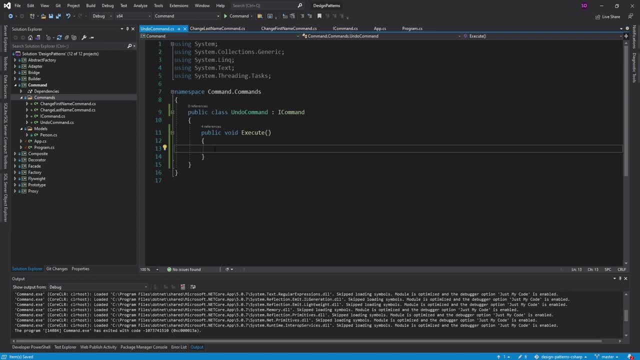 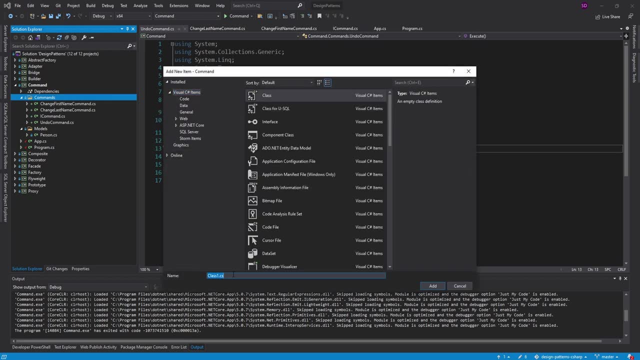 commands are we undoing? we don't have a place where we actually track the commands that have been executed, so we're going to need another class here and this is going to be our command history. so this class is going to track the commands that we've executed so that we know what needs to be. 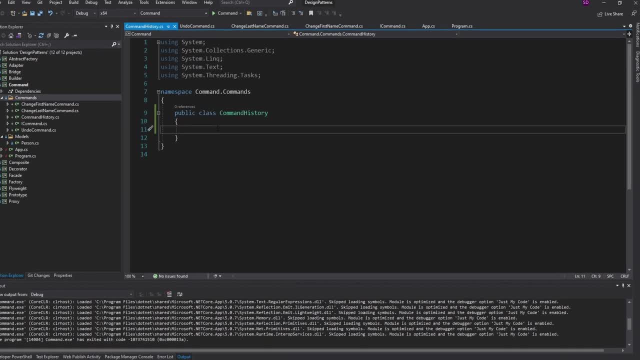 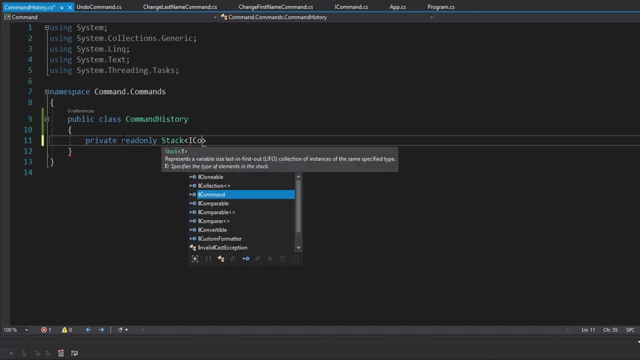 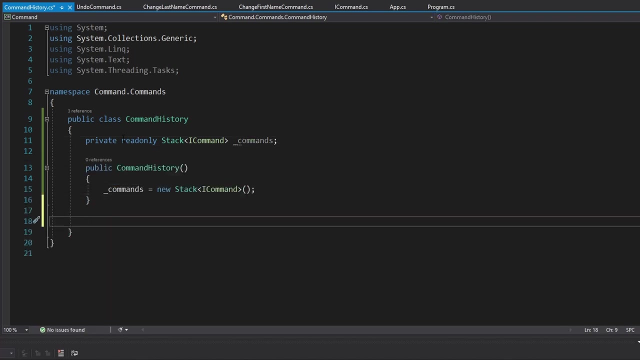 undone and typically to implement history behavior, we would want to use a stack. so let's get a stack field in here. so just a stack that's going to hold our commands that have been executed- and we'll just call it commands- and let's initialize that in the constructor, and in our case, we really only need two methods here. 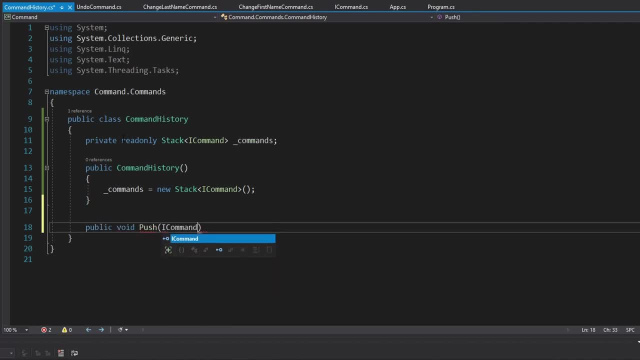 so the first one is going to be push, and this is adding a command to our history. so let's take our command stack and push a command, and then the other method is going to be pop, and pop is going to give back the command that was previously executed, so it's going to pop a command off the 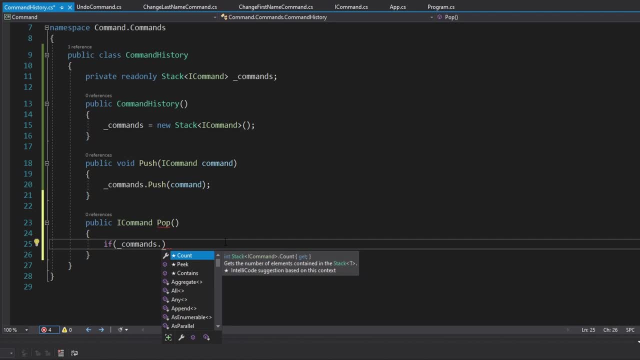 stack, but if there's no commands in our history. so that means our command stack is going to be returned null, and if the command stack has a count of zero, then we're going to actually return null. but if we do have a command in our history, then we're just going to pop it from our stack. 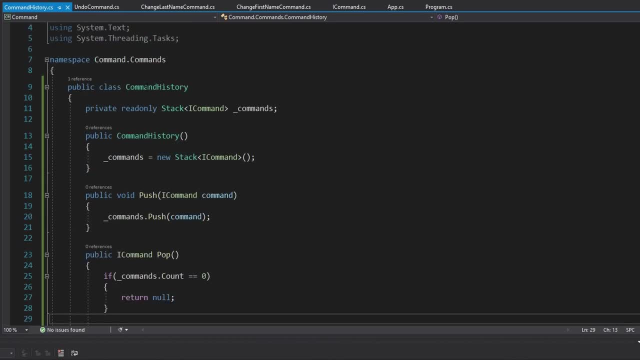 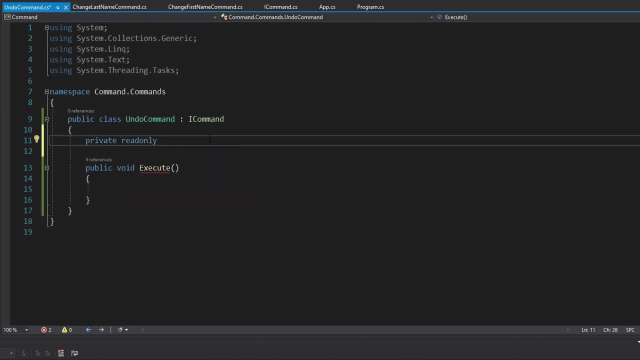 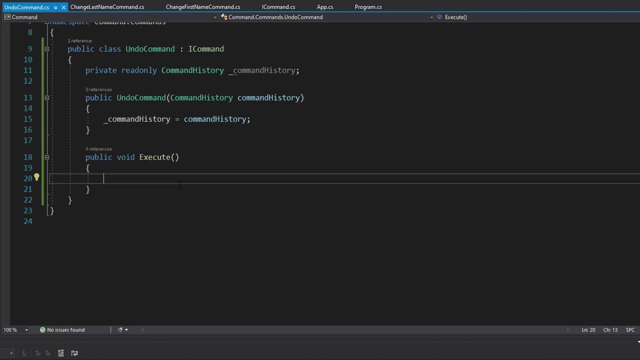 and return it. so let's go ahead and use this command history class inside of our undo command. so we should be done with that. let's get the command history passed into our undo command. so command history: get that through the constructor and when we execute the undo command first, we're. 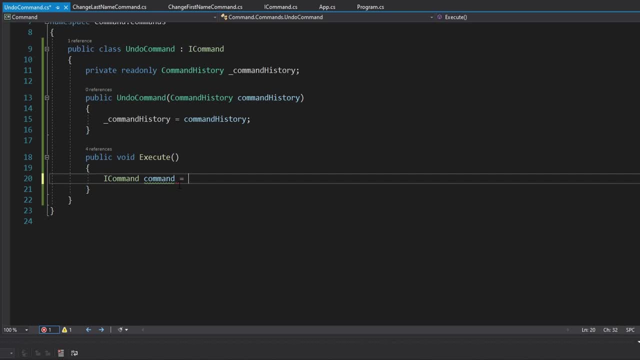 going to grab the last executed command from our command history and we're going to pop it from our command history. so, using command history, pop and then we're going to take that command and undo it. but we actually don't have an undo method on our i command interface. but at the same time i don't 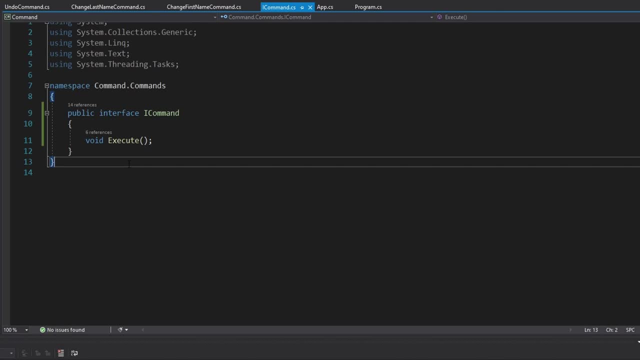 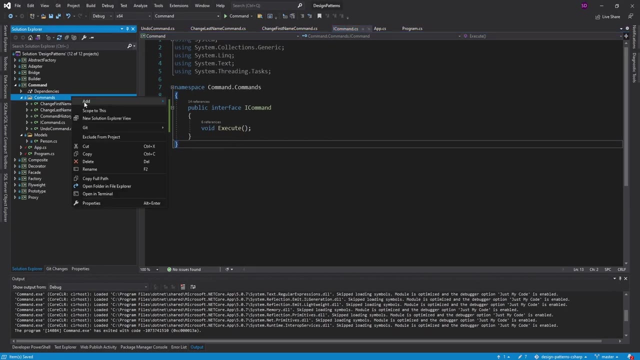 want to add the undo method to our i command interface because i feel like that's enforcing too much on that interface and maybe not every command can be undone. so let's create a new interface and we'll call this the i undoable command or maybe just i undo command. i feel like 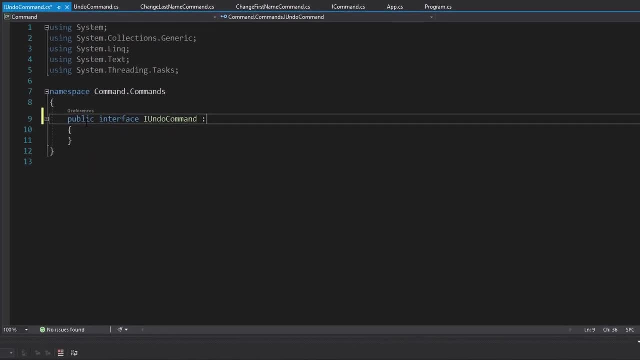 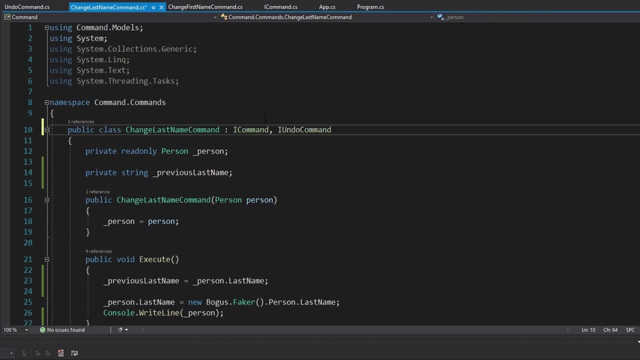 undoable is a little bit excessive and i feel like it's fair for this interface to inherit from i command. and now, on this interface, we're just going to have a single method to undo the command, and now we can use this interface on our existing commands because they can be undone. so this is. 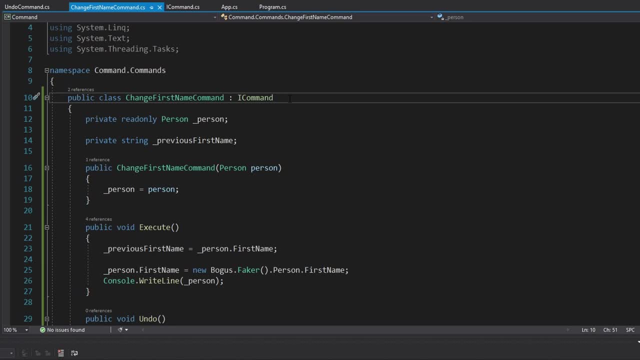 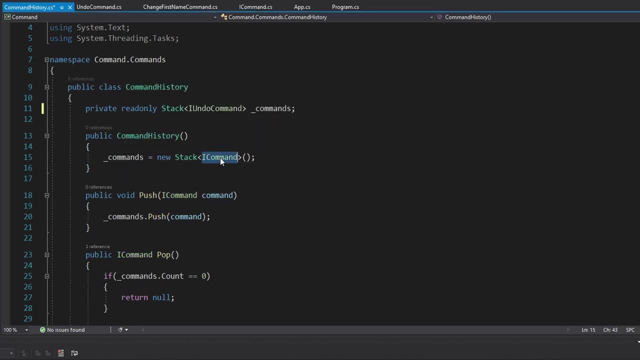 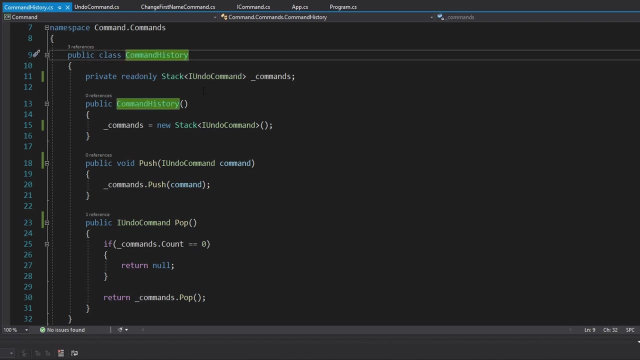 an i undo command and same for the change first name command. we implement that interface and now we're going to change our command history class to take an i undo command instead. so there we go. and now this is a little bit weird because this class is command history, so really it shouldn't. 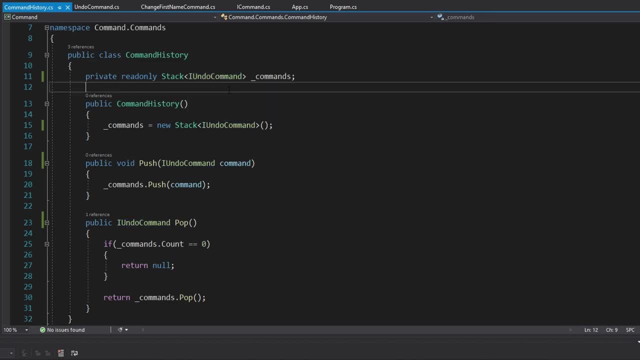 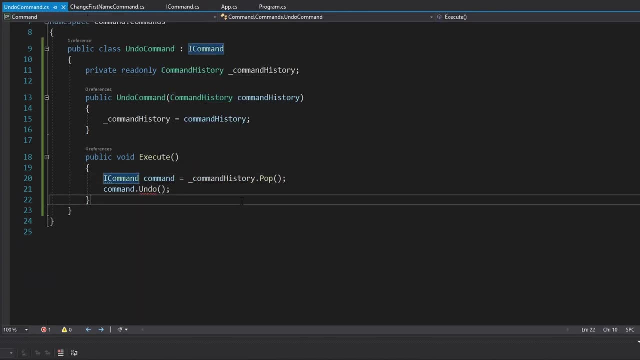 have a constraint on only taking in undoable commands. but for the sake of this demo, i'm going to roll with this implementation. maybe i'm just being too picky, but anyways, back in our undo command. the popping on command history gives us back an i undo command and now we can actually. 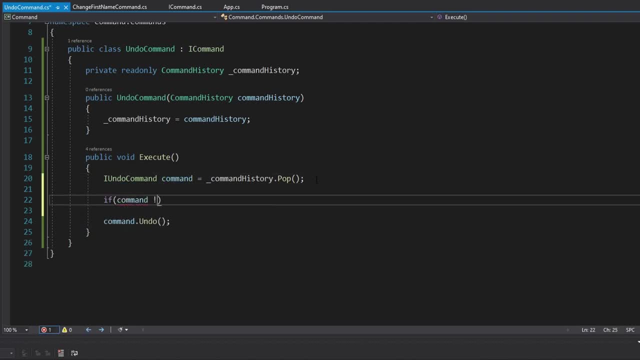 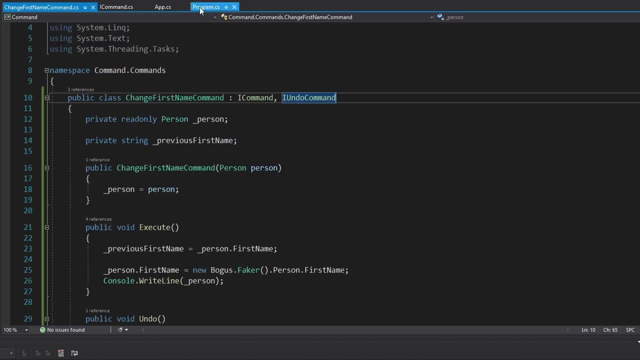 undo it. but we do have to check to make sure that the command does not equal null, and we can really just do that in command undo by using optional chaining. so if the command is null, then we're not going to try and execute undo. all right, the undo command is looking good, so we should be done there now in our programcs. 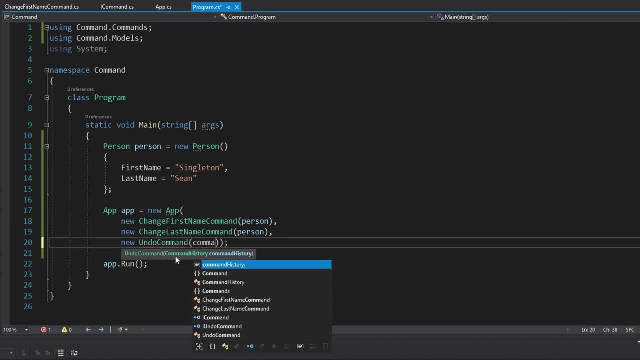 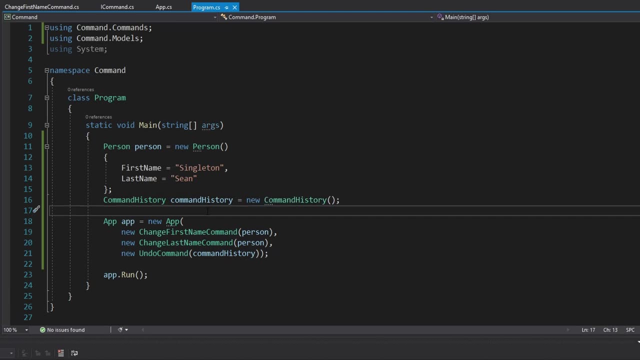 let's pass in the undo command here and we're going to pass in some command history, so let's generate that variable and instantiate that up here, and that should be good. the only issue is that we never actually push any commands to our command history, and this is going to be a little. 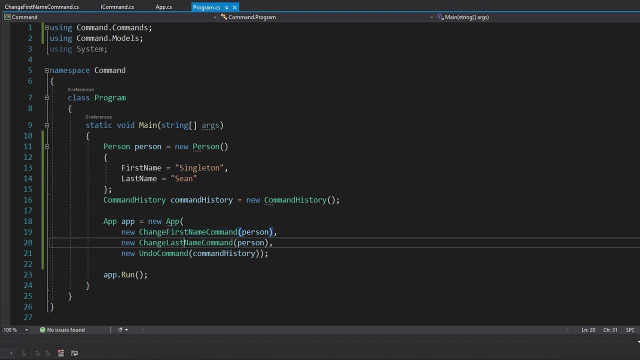 bit weird, but i think i actually want to do this inside of these individual commands. realistically, it might make sense to have like another layer of commands that you would pass in the command history, but i feel like we can make this work and we might even be able to show off some other patterns along the 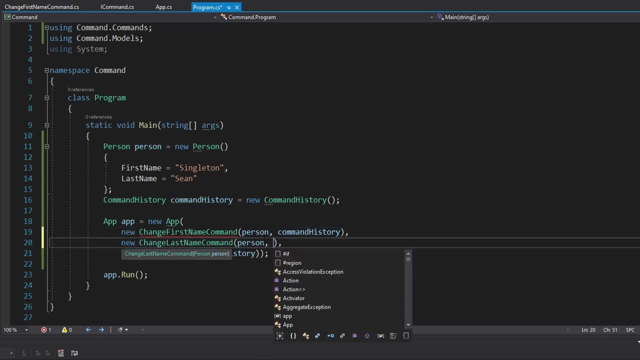 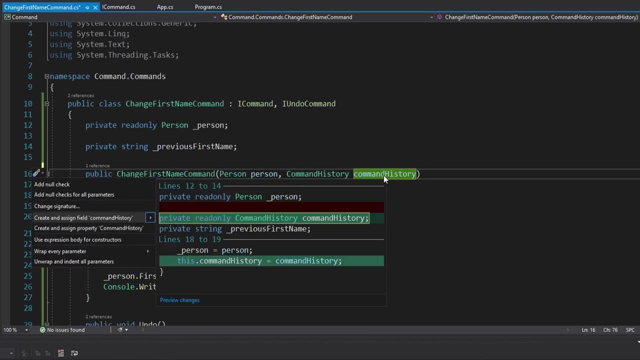 way. so we're going to pass in command history to each of these commands. let's update these constructors, add a parameter to each of these and let's throw command history into a field on each of these commands. so i'll do this for the change last name and last name of each of these commands. 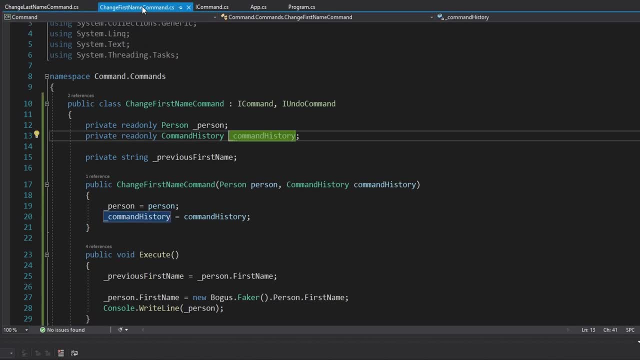 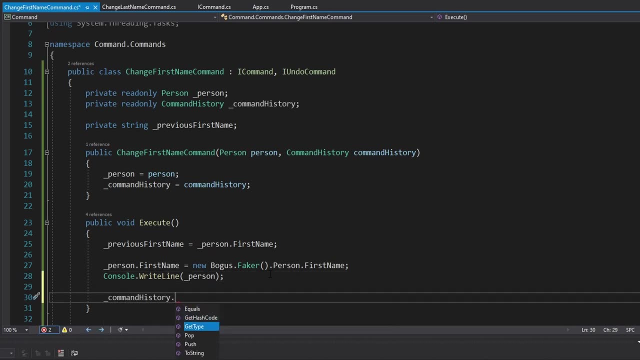 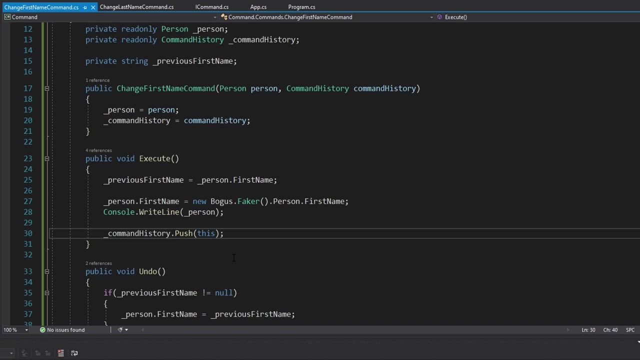 as we go and there we go. now we got command history in each of these commands. so after we're done executing the commands, what i'm going to do is take our command history and push this command so i could just pass in this instance. that's perfectly fine. the only issue is that the next 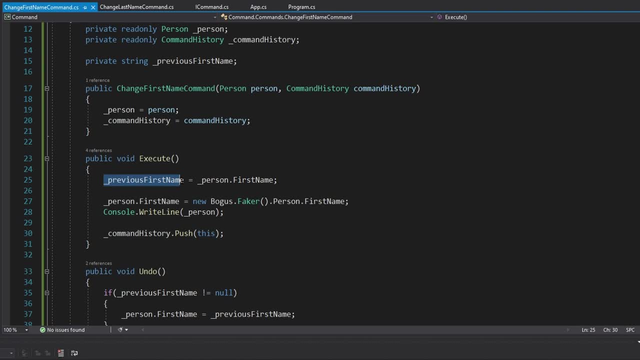 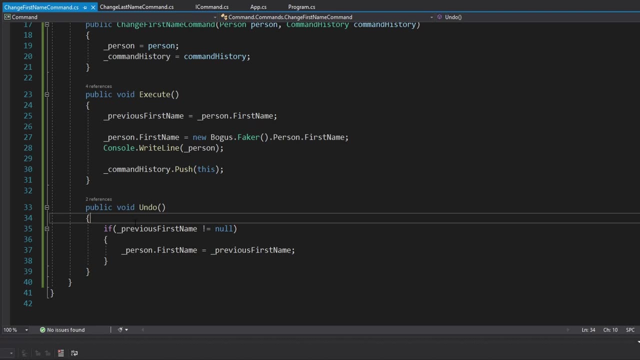 time we execute this command, we're going to overwrite the previous first name and that means whenever we undo, we're not going to be undoing what we did before, and actually maybe we're going to be understanding how to do this kind of thing- probably not Because different. 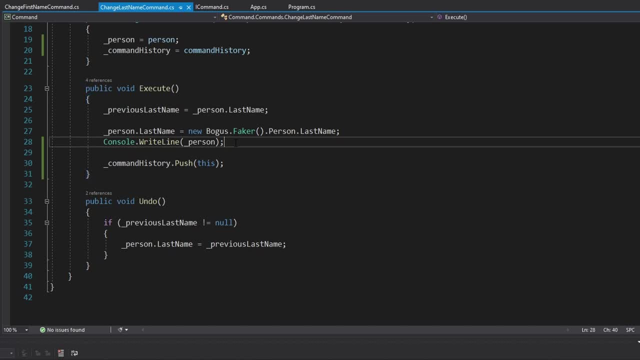 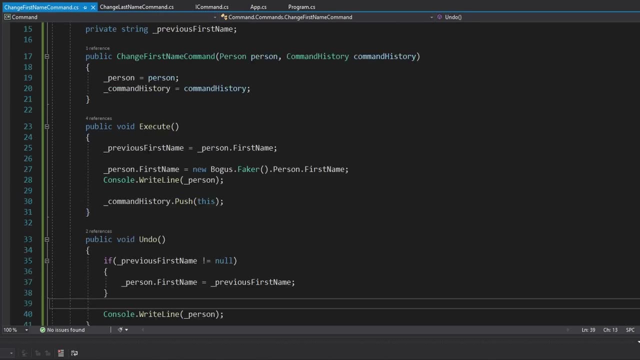 guys. it depends on the yo theft. they don't always have a bear that's just going to believe their kind of options. we're not playing with flow. we're just going to be seeing how do we do this if the more ways of doing that. but i'm just going to use my command history to pass in the. 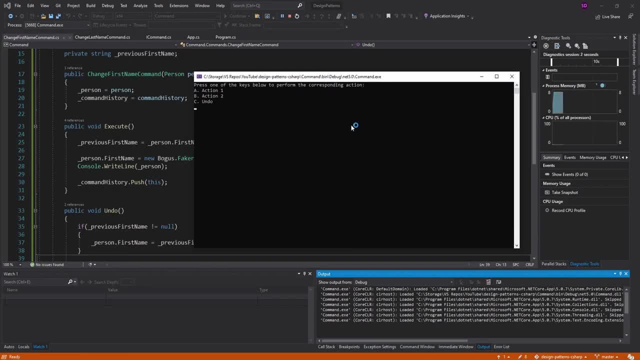 command history toéro: create command history and after that i'm just going to change this to something i key know this list- then after that i'm going to just move this command history to create the code- a little bitiguar, just in case. i'm not sure how this works, but you know what like. 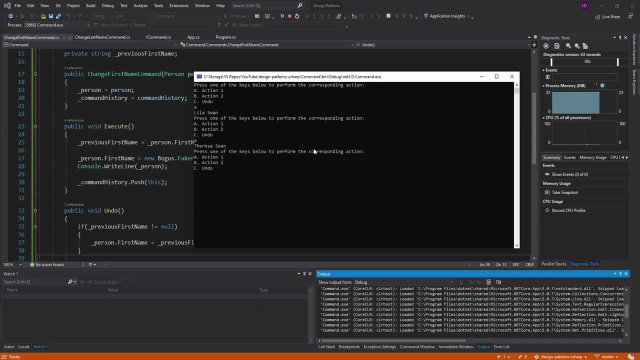 what's driving today to怎么? a lot of times like i'm not sure, probably in particular when a co制, philip james and let me do command history- push in the change last name command as well, and then again, and now we're Teresa Sean. And now let me undo, So, undo, successful. we're Lila Sean. now. 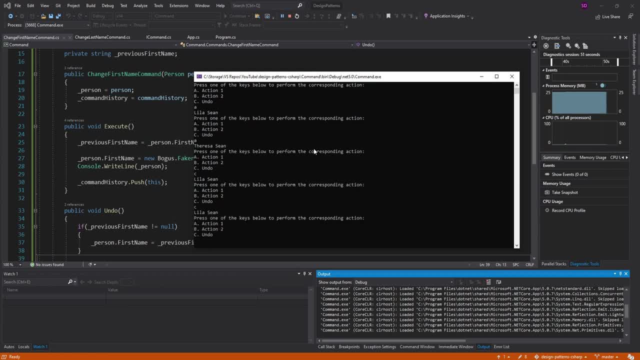 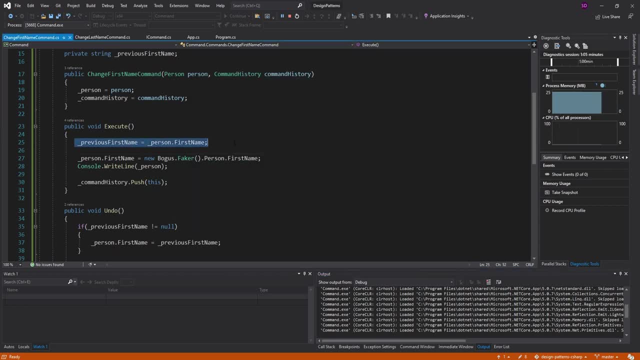 that's as expected. But now undo again and we're still Lila Sean, And the reason for that is because whenever we changed from Lila Sean to Teresa Sean, we overwrote the previous first name from Singleton to Lila, And that's because everything is happening inside of this single. 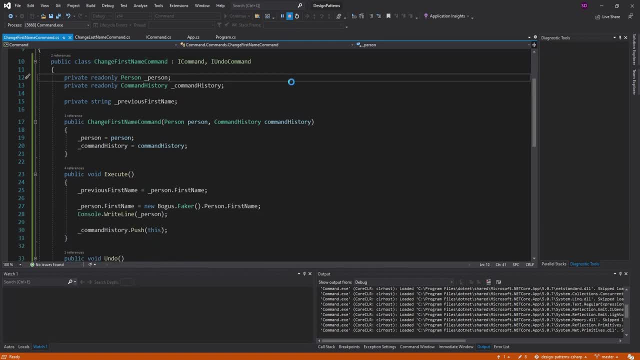 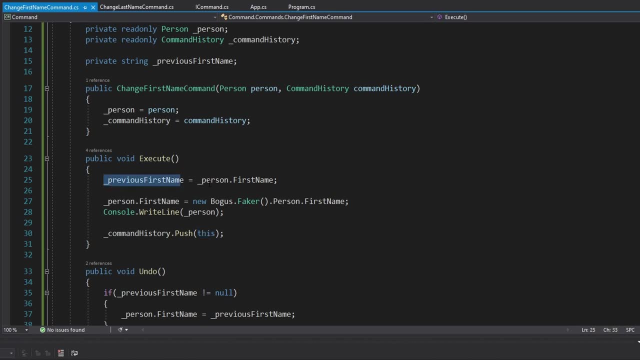 change first name command instance. So what we should be doing is cloning this change first name command and then pushing it to command history so that we don't overwrite the previous first name. So cloning. what pattern do we use for that? I'll give you three seconds to guess, Okay. 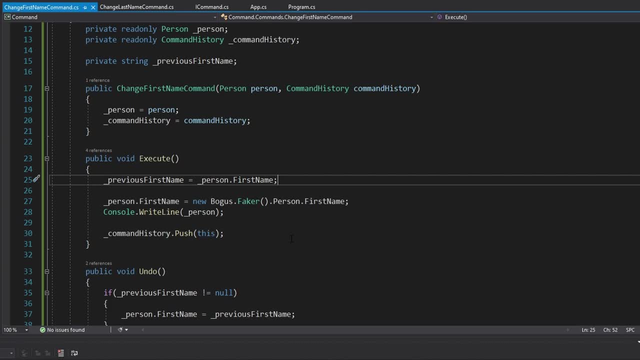 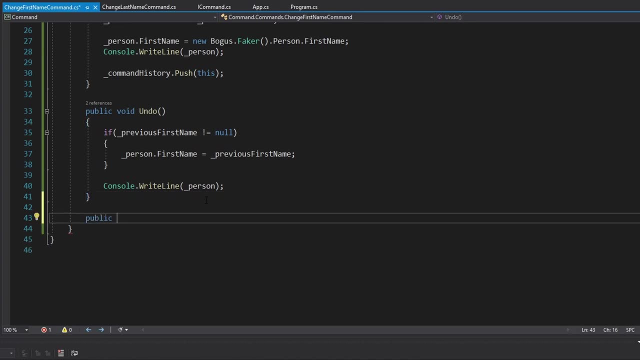 three, two, one prototype, Oh yeah. Okay, we're gonna use the prototype pattern to clone our commands. So we're gonna have another method on here And actually doesn't really have to be public and just be private, Because we're doing all this inside of our command. So I don't even know if this qualifies. 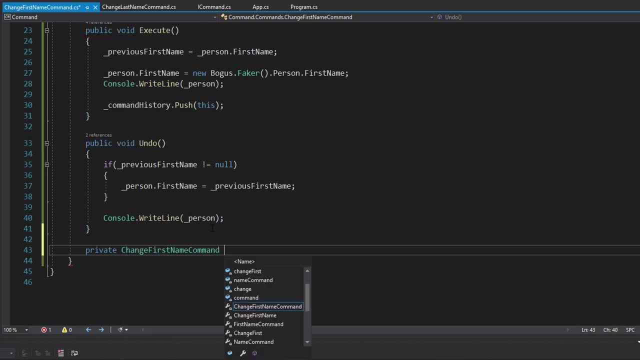 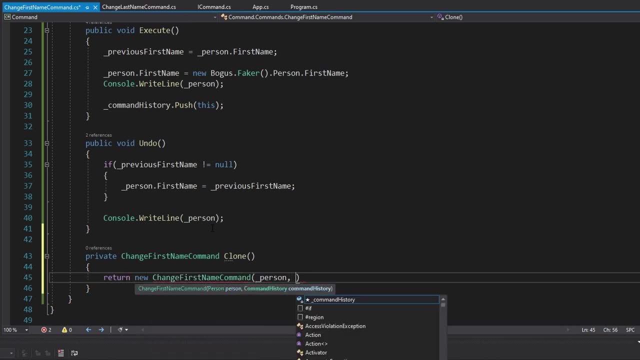 as the prototype. but we're going to return a new change first name command instance And I'll just call this clone. And inside here we're just going to return the new commands. we're going to pass our person in here, pass our command history in here And actually we have to set previous first. 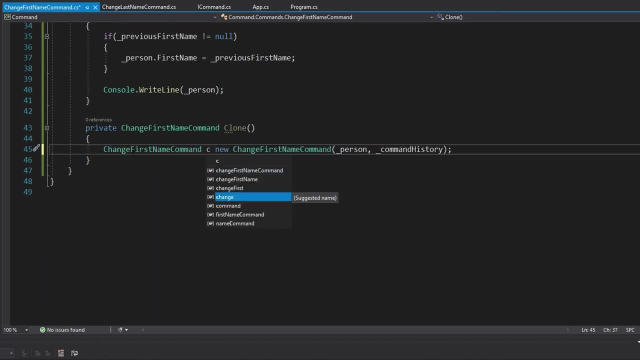 name to what it is currently. So let's put this into a variable first, and then we'll end up returning it. But in between here we have to set the previous first name. So let's call this clone to whatever the previous first name is at the moment. And now since. 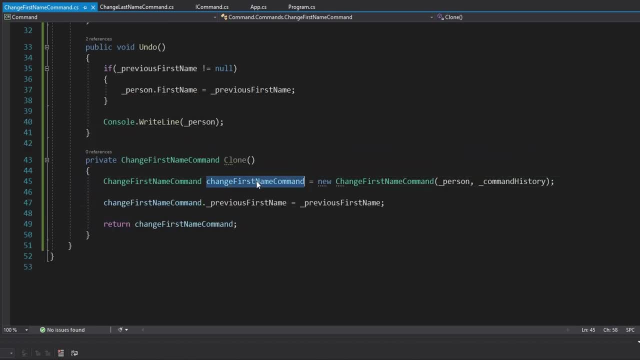 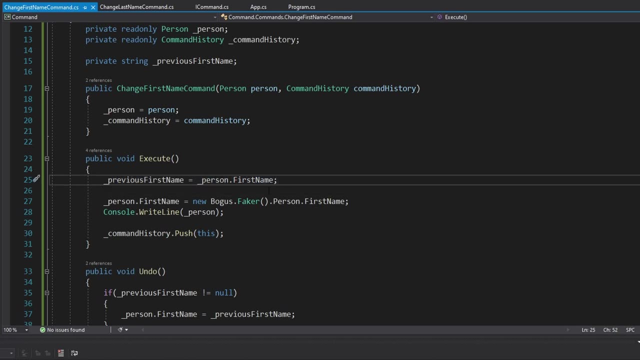 previous first name is on this new instance and this is going to get passed to our commands history. that means we can change previous first name on the next execution And it's not going to mess with our commands history, So let's push this clone into here. So instead of passing this, 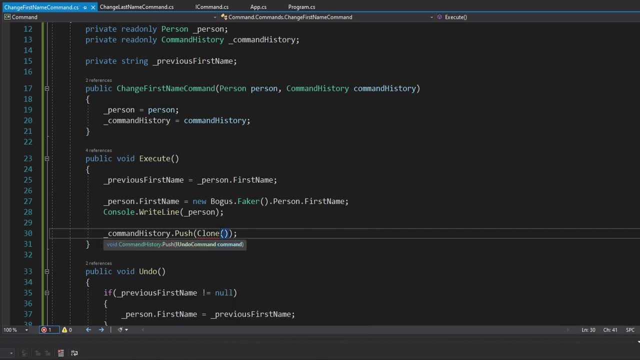 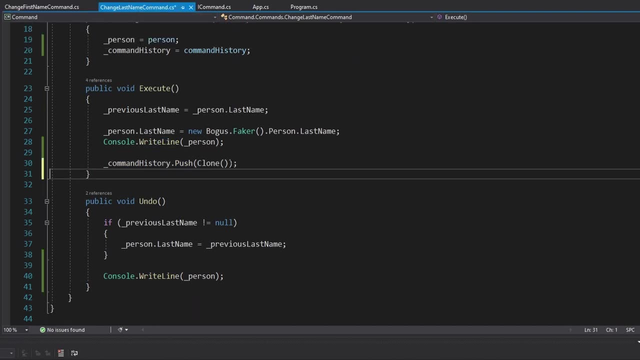 we're going to pass the clones commands. So call clone, get our commands back and pass it to command history. And we're going to do the same thing for the change last name command: pass in a clone. let's get our clones in here. and this is the change last name command now. so let's. 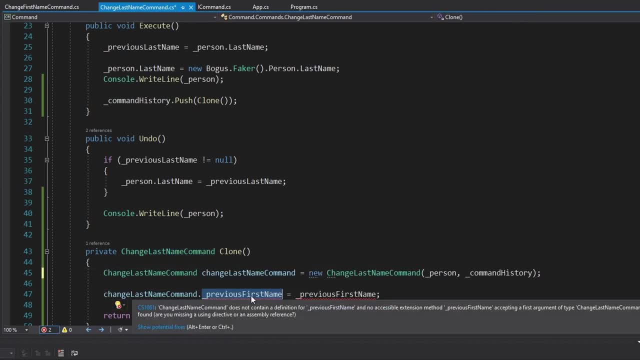 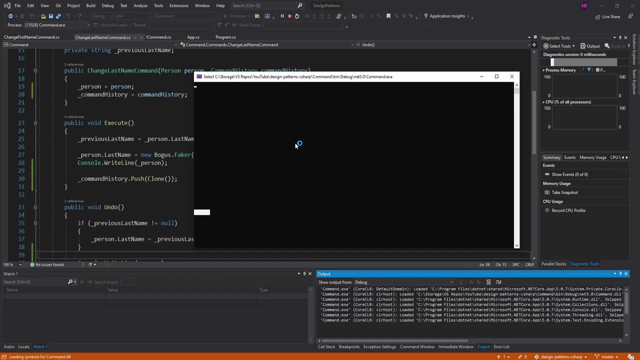 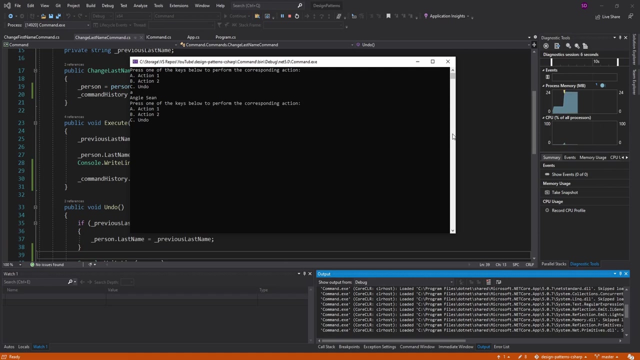 make sure we change that everywhere so that it makes sense and we're setting the previous last name to the current previous last name. all righty, now we're gonna run this and we should be able to undo as we expected. all right, so change first name. there we go. we got angie sean, change first. 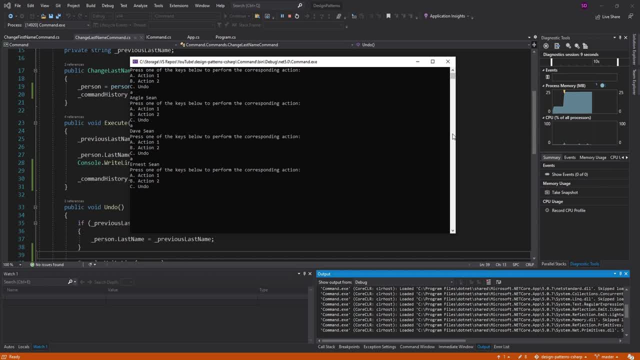 name again: dave, sean. let's do it one more time: ernest, sean. and now let's undo all of this. so we should go back to dave and then to angie and then to singleton. perfect, that works as expected. and now let's mix in some last name changes. so let's change first name. first we got inez sean and then 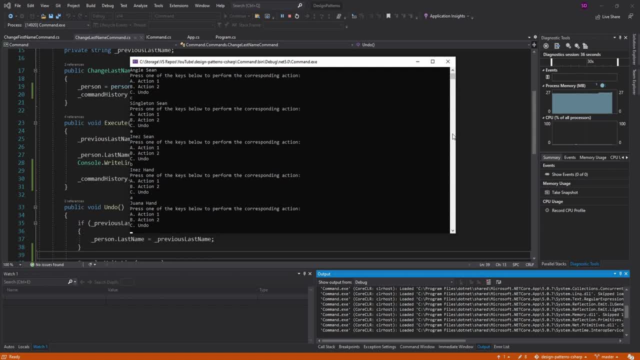 change the last name- we got inez hand. change first name- we got wanna hand- and then change the last name wanna turcotte. all right, let's undo all of this until we get back to Singleton. Sean, Here we go. Cool, That was awesome. I didn't. 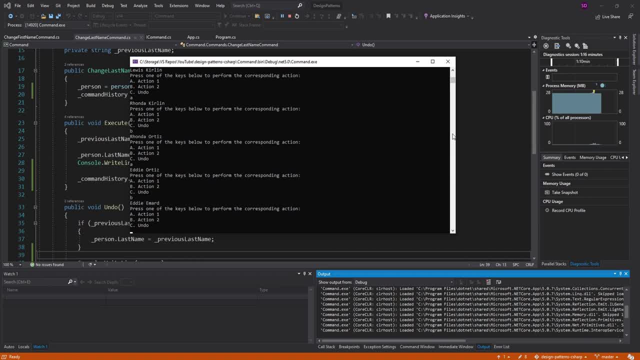 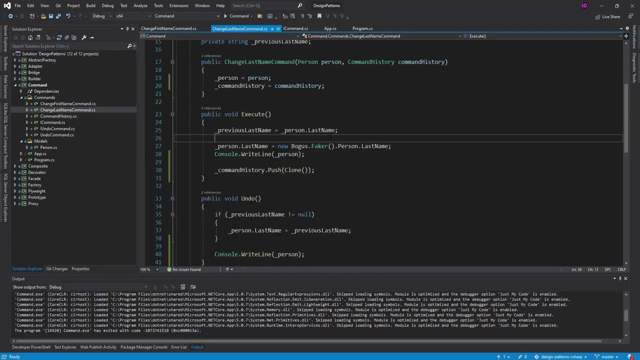 think of that. We can just spam these buttons as much as we want and then hold down C, and we eventually get back to Singleton Sean, which is somewhere up here. There we go. So it looks like our application is working as expected, but, most importantly, we have implemented the command. 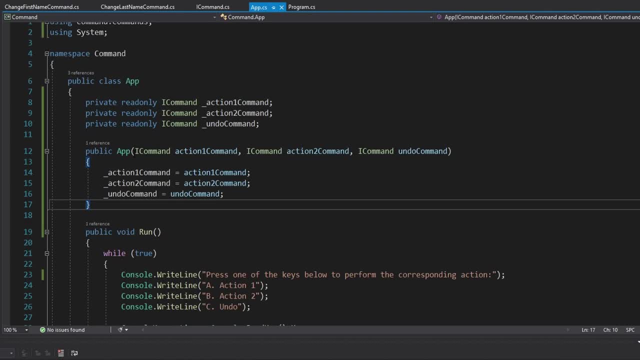 pattern. So let's review this. Our user interface depends on these I commands, which means any other application could reuse this user interface. All they'd have to do is pass in the commands that they desire for their own application and our user interface would support it as long as they. 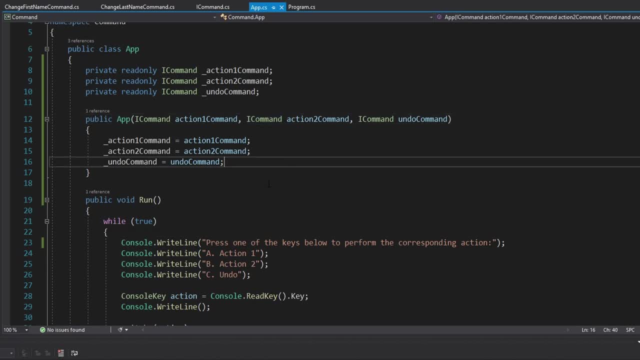 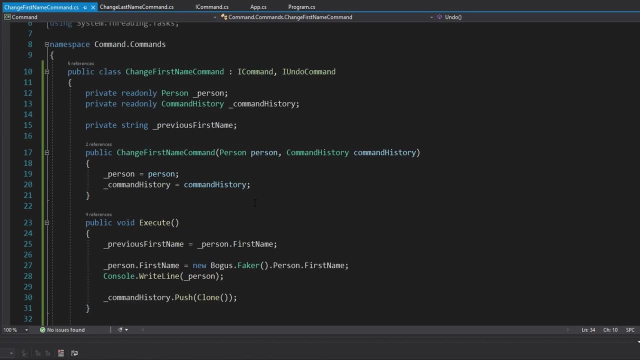 implement the I command interface. And then the other fun thing that we showed off was the ability to undo commands. So since our operations are wrapped inside of these command classes, we can store additional things, such as the previous state, so that we can support those undo operations. And 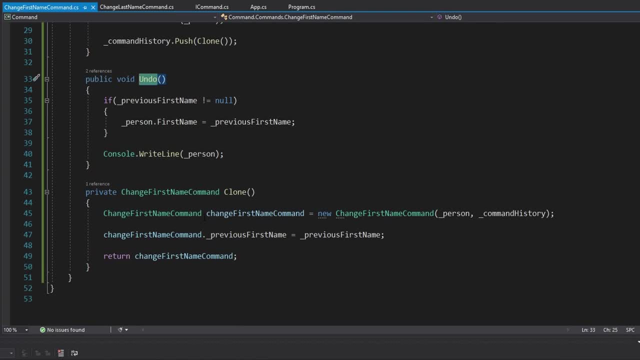 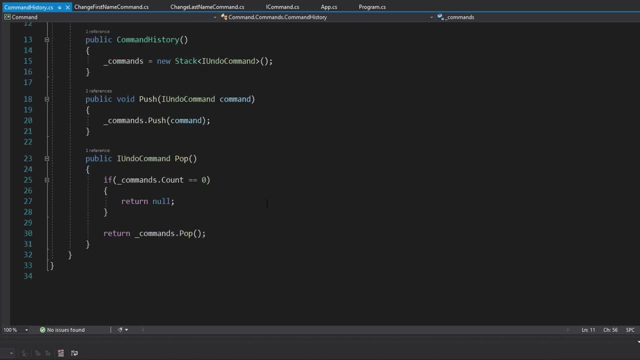 not going to lie, I thought that was a pretty cool demo doing the whole undo thing, So we got to see the prototype pattern kind of. and then we did some cool data structures So we got a stack to show off our commands, history, And yeah, that's pretty much it. Maybe it wasn't that. 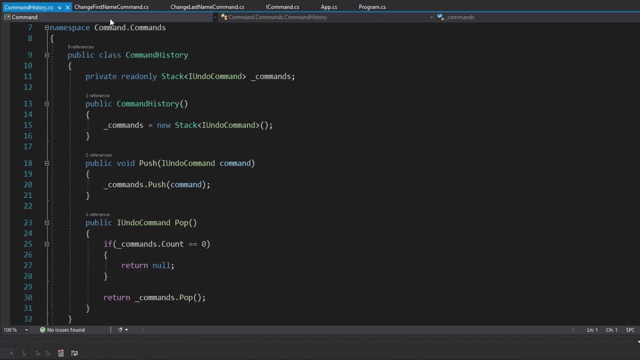 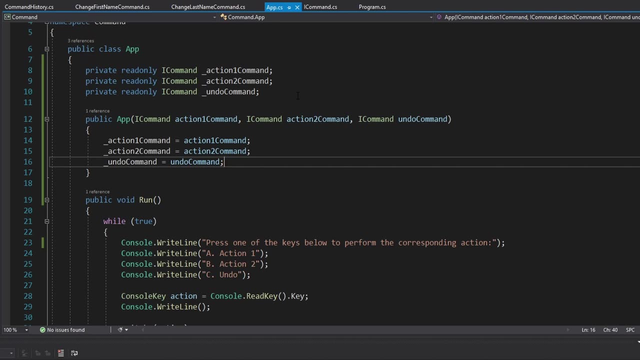 cool, but hey, it did work and we got to see the power of the command pattern. Anyways, hopefully you find the command pattern helpful for your own applications And if you're building UI applications, such as with WPF, you probably already used it and see that it is helpful. But aside from that,